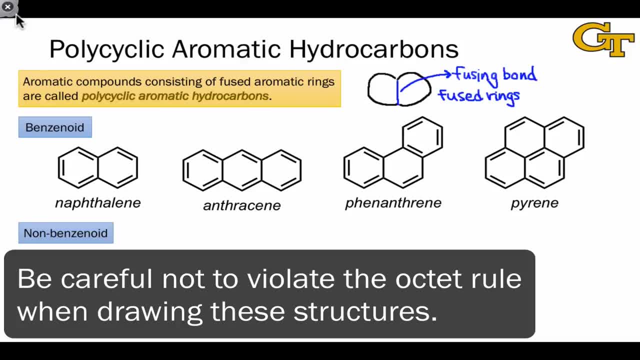 The most important benzenoid polycyclic aromatic hydrocarbons are listed here. All of these are aromatic and they all satisfy the 4n plus 2 rule. Naphthalene has 10 pi electrons: 4 in the ring on the right and 6 in the ring on the left. 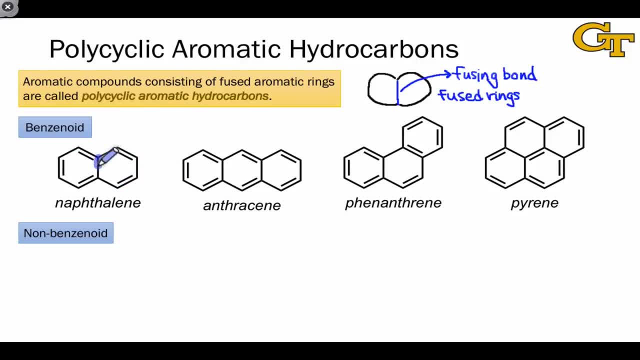 and consists essentially of two fused benzene rings. where the fusing bond is right here? There are actually two ways to fuse another benzene ring onto the structure of naphthalene Fusing to create a linear structure of three benzene rings. using this bond leads to anthracene. 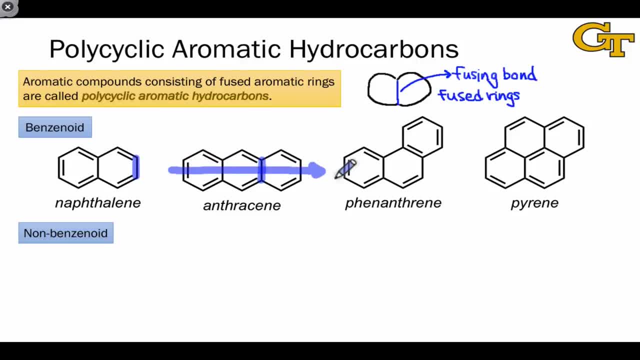 a molecule consisting of three benzene rings fused in a linear fashion. Fusing in an angular fashion using this bond leads to a molecule consisting of three benzene rings fused in a linear fashion. using this bond leads to a molecule consisting of three benzene rings fused in a linear fashion. 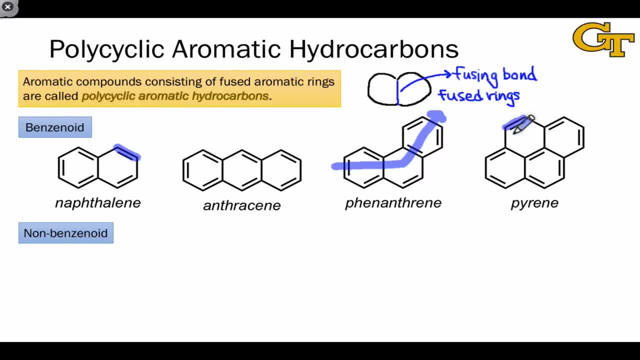 This molecule is an isomer called phenanthrene. Introducing another ring into phenanthrene by adding two carbons that are linked here and here results in the molecule pyrene. All four of these molecules have structures and reactivity that resembles benzene, indicating that they're aromatic. 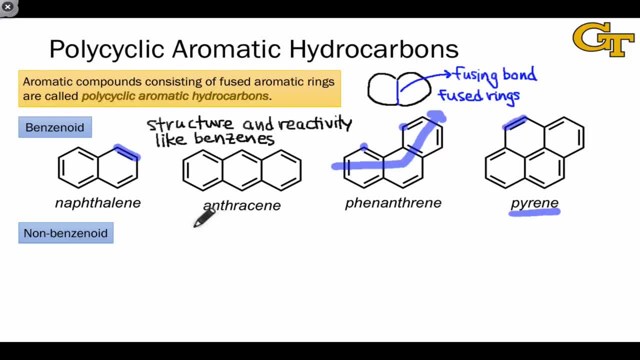 For example, they don't undergo addition chemistry in the presence of electrophiles, instead opting for substitution. just like benzene, Non-benzinoid polycyclic aromatic hydrocarbons consist of ring sizes different than 6.. Two examples are shown here. 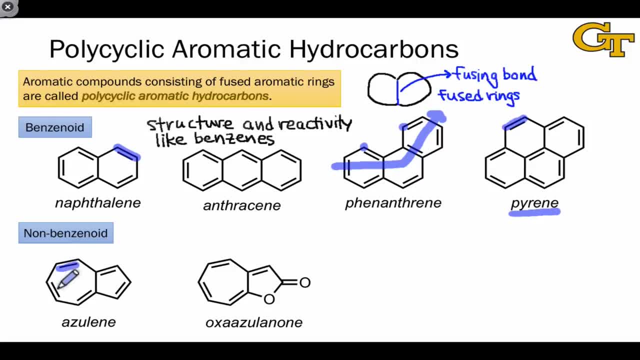 Azulene is a constitutional isomer of naphthalene. Just like naphthalene, the molecule has 10 pi electrons, indicating that it's aromatic. However, this molecule isn't as simple as it looks, as we'll see in a second. 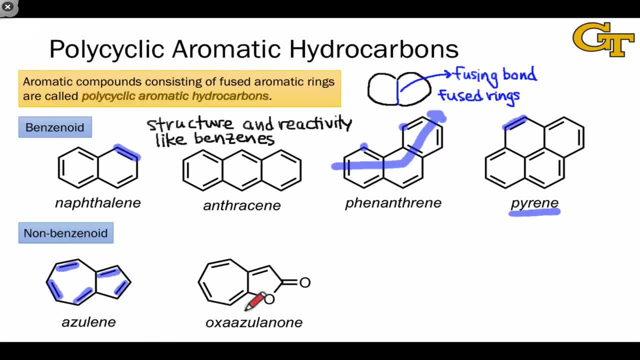 Looking at the second example, an oxygen-containing analog of azulene, we might be hard-pressed to understand how this molecule is aromatic. The key to understanding this molecule is to consider resonance structures involving a lone pair on this oxygen atom within the ring and the CO double bond. 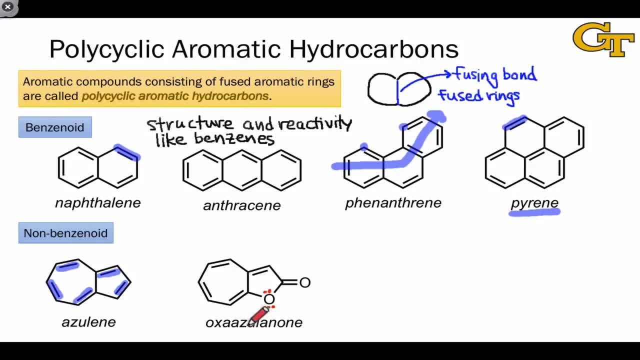 This is actually a common theme when it comes to aromatics-containing heteroatoms that we'll return to in later discussions of aromatic heterocycles. thinking about resonance, An important resonance structure of this molecule involves donation from the oxygen within the ring toward the CO pi star orbital. 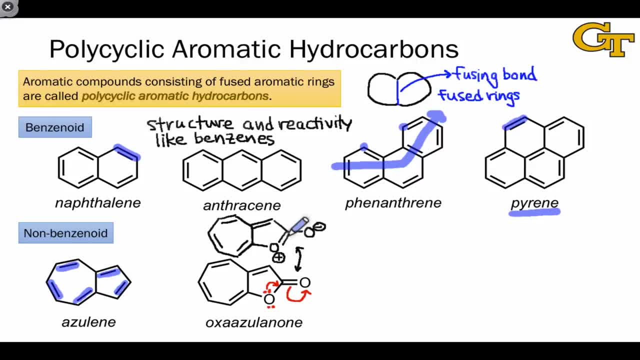 In the resonance structure resulting from this electron flow, we can see pretty clearly that the CO double bond is a monomer. This means that the molecule has 10 pi electrons, corresponding to the 5 pi bonds within this resonance form. The fact that this resonance structure appears aromatic indicates that it's probably very important to the overall structure of this molecule. 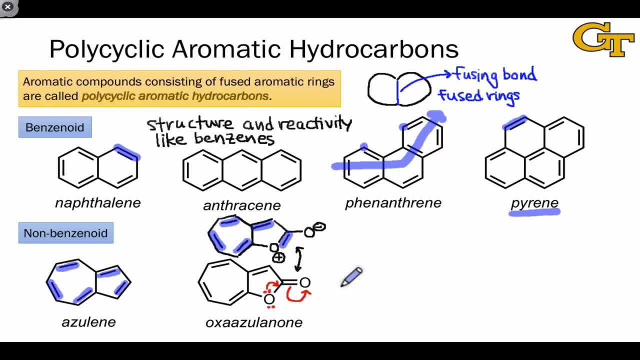 The importance of this resonance structure gives us structural insights. For example, since this resonance form is aromatic, we might expect this oxygen to be more negative than the oxygen of a simpler non-aromatic ester, something like ethyl acetate or something with just a plain vanilla alkyl ester. 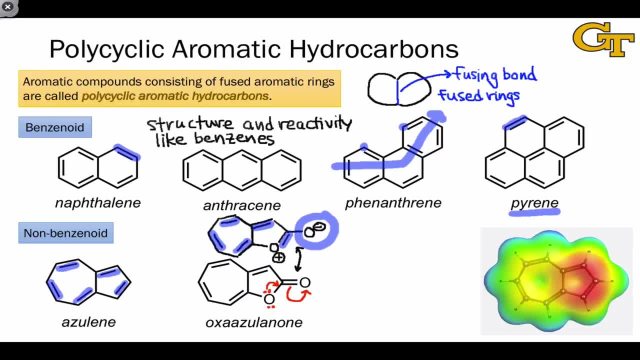 A related idea comes up if we look at the electrostatic potential map of azulene. If we were to look at azulene from a sort of classical introductory chemistry perspective and ask whether this molecule is polar or non-polar, it appears completely non-polar because it's made up of C-C and C-H bonds, none of which are strongly polarized. 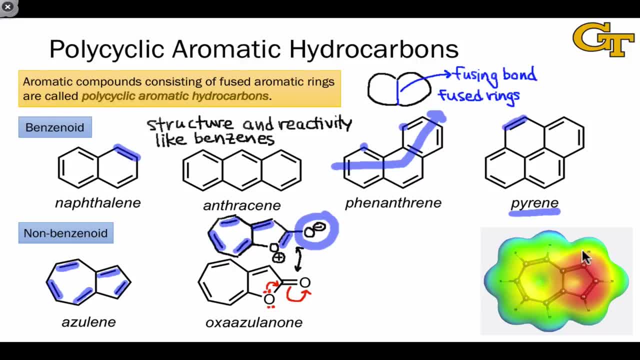 However, if you look at the electrostatic potential map of this molecule, we see that it is actually heavily polarized, with the 7-membered ring having much less electron density than the 5-membered ring. What's going on here? 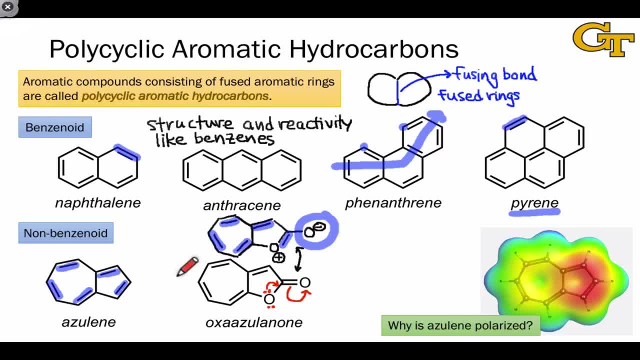 Why is this molecule so polarized? Well, again, resonance can come to our rescue here and help us understand why this polarization leads to a stabilizing effect in the molecule. Consider a resonance structure in which I push pi electrons to shift charge toward the 5-membered ring. 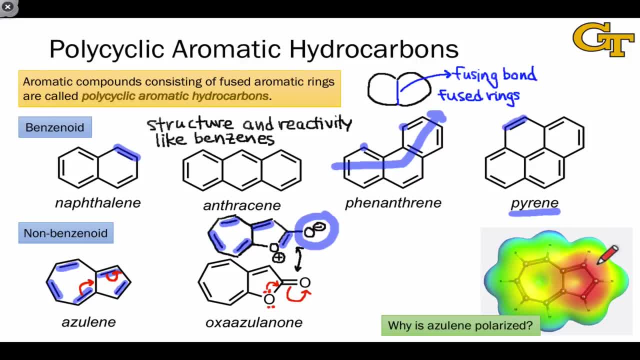 Electron flow like this is indicated by this electrostatic potential map, since the right-hand side of the molecule, the 5-membered ring, appears more electron dense, more electron rich than the left-hand side. This electron flow leads to the resonance structure that I'm drawing here. 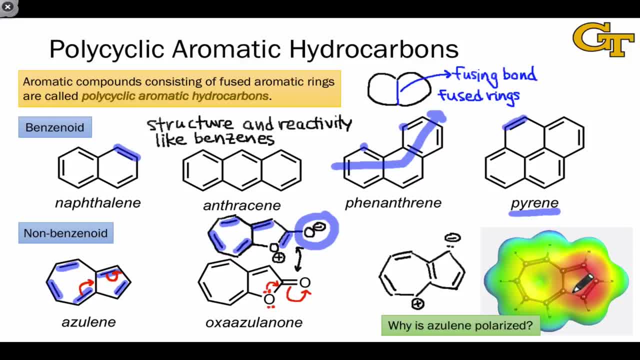 And clearly this resonance structure is a pretty good representation of the molecule as a whole, since it illustrates the electron-rich nature of the 5-membered ring and the electron-poor nature of the 7-membered ring. But what's so special about this resonance form? 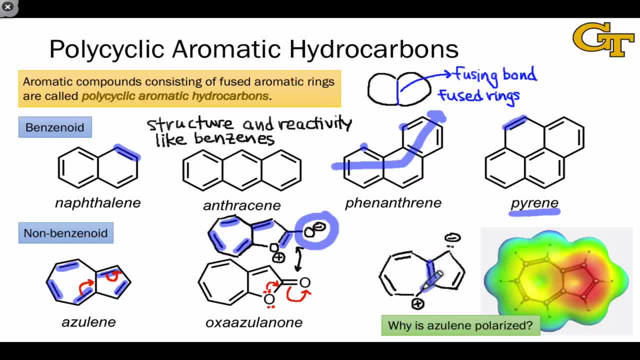 The thing to notice here is that if we look at each of the rings individually, each of the individual rings is aromatic. So I'm highlighting the 7-membered ring first and notice that we've got a cyclic structure that's fully conjugated with 6 pi electrons. 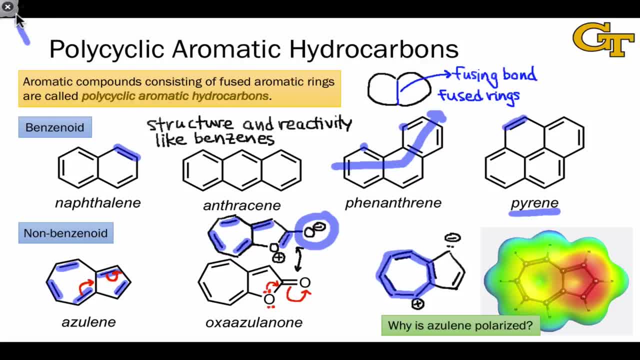 2 due to each of the pi bonds. That's an aromatic substructure within this molecule. Let's consider the 5-membered ring separately. now I've got a 5-membered ring that is fully conjugated. it's, of course, cyclic, it's planar. 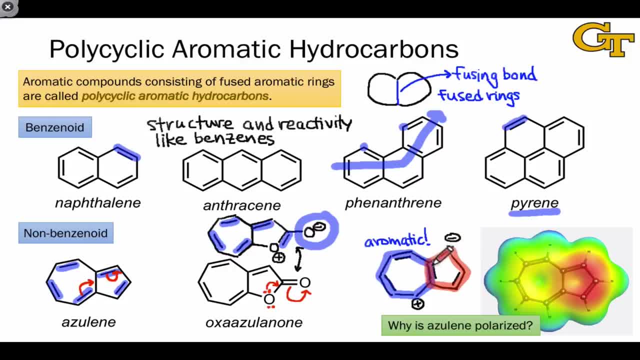 and it contains 6 pi electrons: 2 due to the lone pair and 2 each due to the pi bonds. This substructure within the molecule is also aromatic. What this analysis helps us see is that this polarization stabilizes the molecule by creating two distinct aromatic systems. 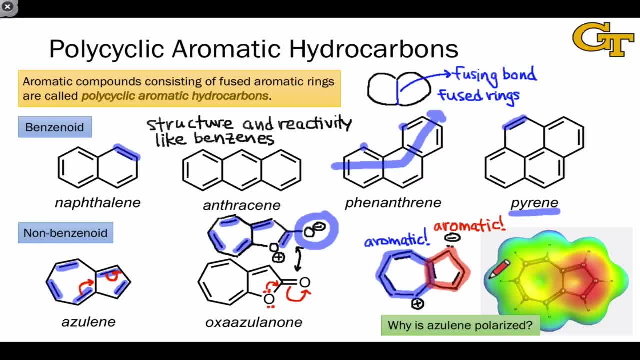 This results in an aromatic stabilization energy that's greater than it would be in the absence of this polarization, And you can see the polarization in the shapes and occupancies of the molecular orbitals. So far we've been talking about cyclic fully conjugated hydrocarbons. 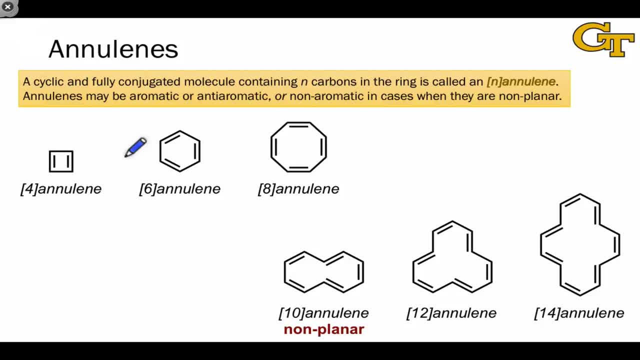 which have this pattern of alternating double and single bonds- And- that's kind of a mouthful to say- cyclic and fully conjugated. every time There is a term that's been invented to refer to these cyclic fully conjugated hydrocarbons. They're called anulenes. 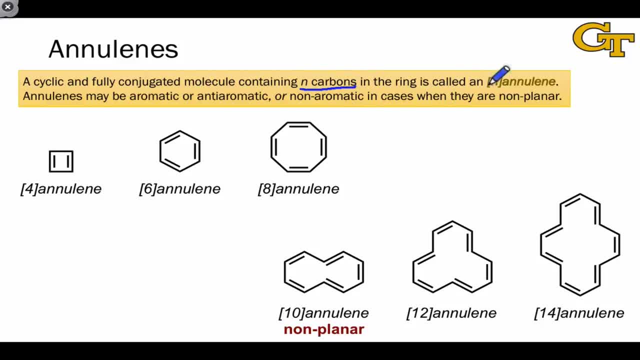 An anulene containing N-carbons within its ring is called an N-anulene, with the N in brackets indicating the ring size. Depending on what criteria of aromaticity they satisfy or don't satisfy, anulenes may be aromatic, anti-aromatic or even non-aromatic in cases when they're non-planar. 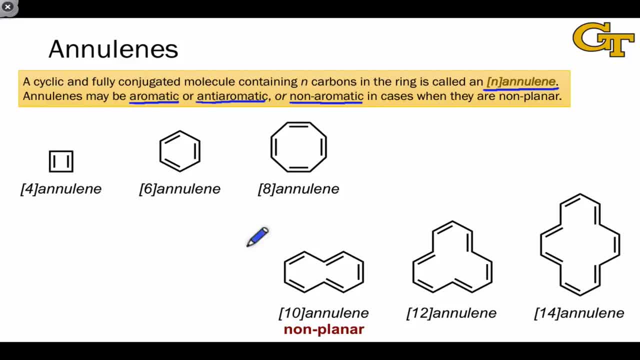 which comes up due to steric hindrance in some cases, or to avoid anti-aromaticity. We can think of cyclobutadiene, benzene and cyclooctatetraene, three molecules that we've talked about, but they're not aromatic. 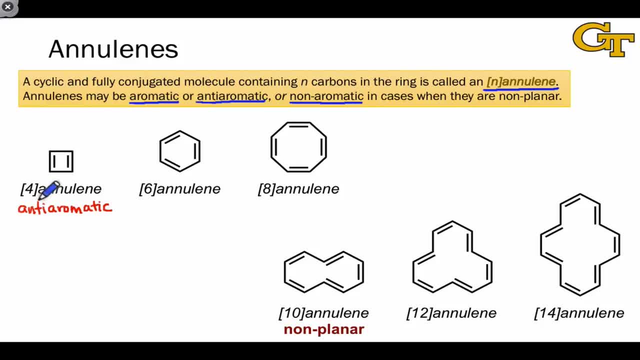 We've talked about them previously as anulenes in their own right. Cyclobutadiene is anti-aromatic due to its 4 pi electrons, while benzene is aromatic, while cyclooctatetraene is best described as non-aromatic. 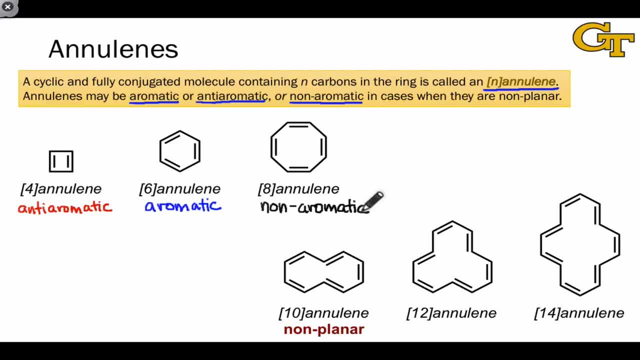 because, although the molecule would be anti-aromatic were it fully planar, in actual fact the molecule is non-planar. This 10-anulene is in a similar situation and this one's remarkable because it would be aromatic right. 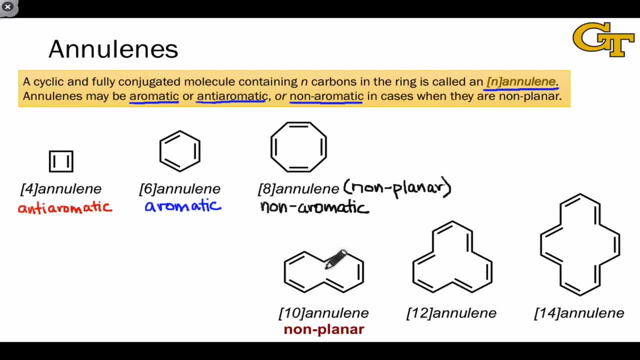 It has 10 pi electrons, so it would be aromatic, but the molecule is non-planar and it's forced to be non-planar due to the orientations of these hydrogens, which I kind of have to draw in in a strained way just to show them distinctly.